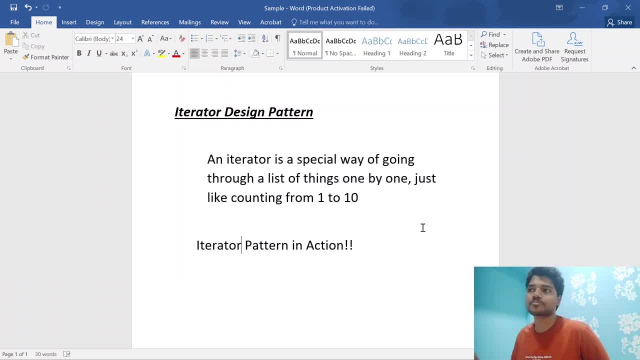 Or the other way is, like by by calling a function called iterator. So you will. you're asking like iterator, hey, iterator, this is my data, just take my data and and just give me the data in a sequential way, like So: I don't want to access my data through indexes, through indexing, through get operation. 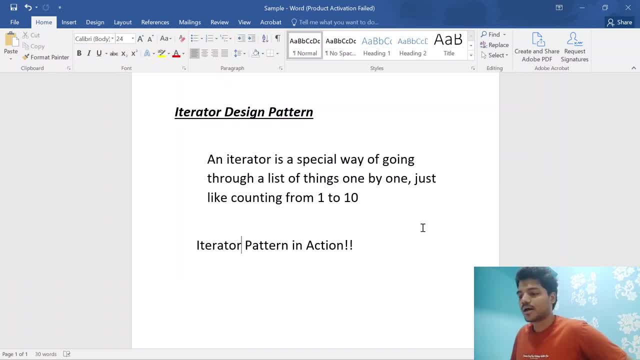 So likewise like iterator will be helpful. So that's exactly how iterator works like. So if you have furlough from i equals zero to ten, with a single uh increment operation, it will basically print one to ten, right? So in a sequential way, like in: 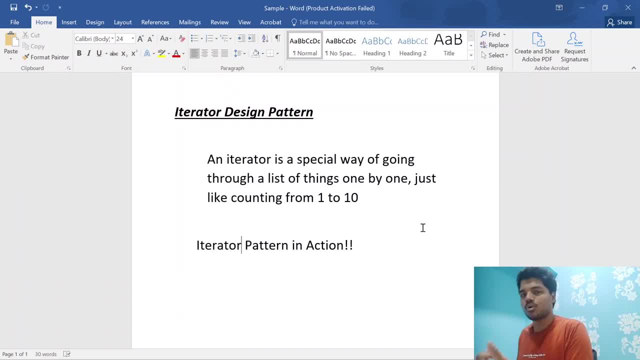 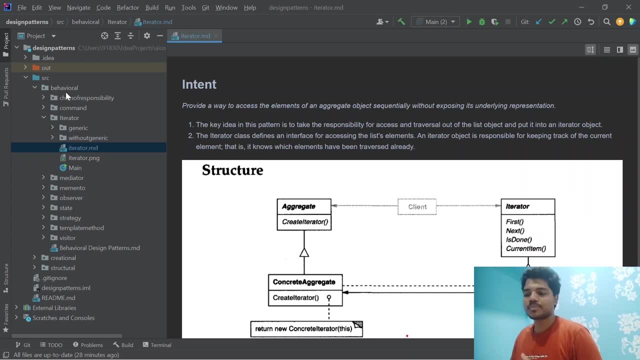 a uniform way, that uniformity is a most important concept here. like Now let's see this definition and then we can go through multiple examples. So because of iterator is small concept I have, I have given multiple examples to get more idea. like: So iterator is a provider way to access the 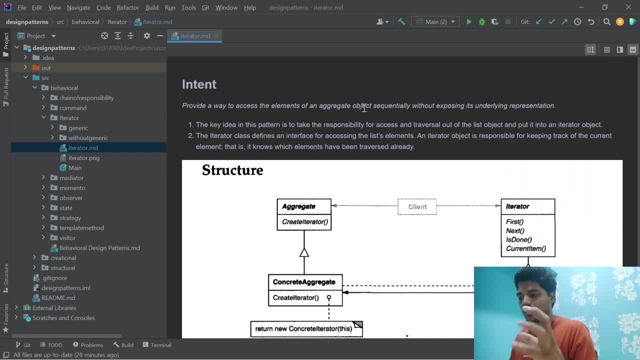 elements to an aggregate, an object of an aggregate. object of an aggregate of the sequentially- This is the most important- without exposing its underlying operations. So it will, uh, whenever asking what is the next value, it will just, it will simply give. you don't even know what exactly inside there, like, If you ask next, it will give, it will give the next. 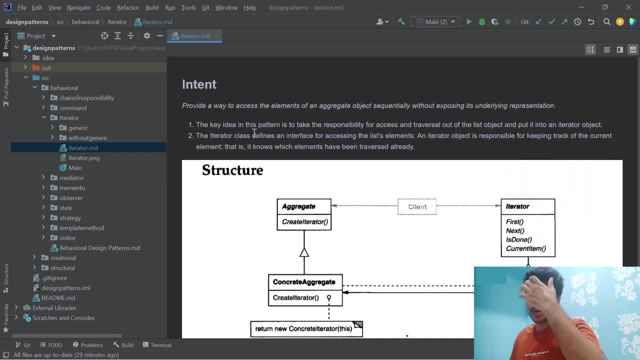 value like. That's how iterator will basically works. The key idea in this pattern is to take the responsibility of for for accessing and traversing of out of the list object and put it into the iterator object. I already discussed right. We are handing over our uh iteration. 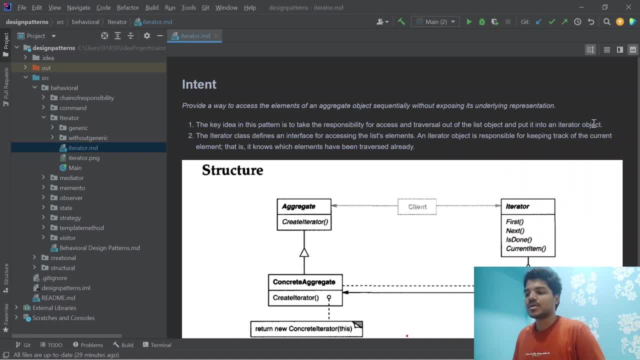 task to the iterator object. like So all the traversing task. So the iterator object will basically take care. like So iterator object is responsible for keeping track of the current element. So the here the most important thing is sequential, So it needs 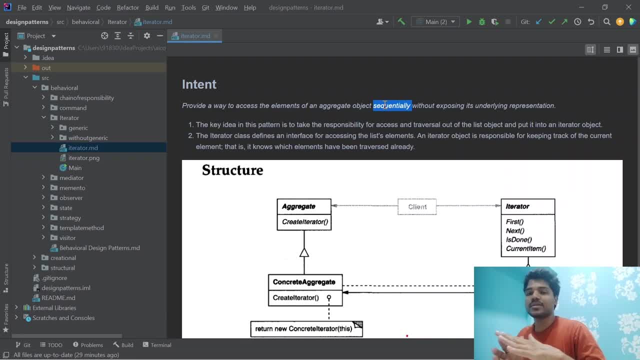 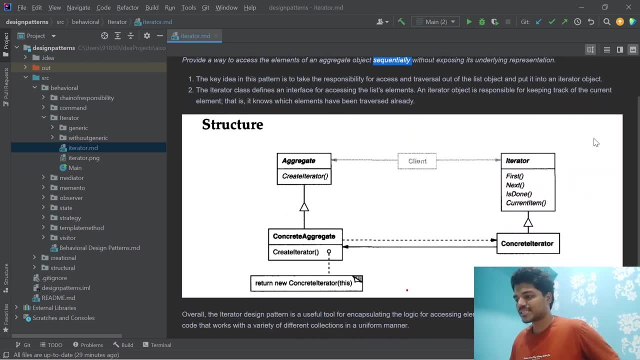 to keep track the previous elements, uh, the current element, so that it will give the next element, only it will not give some other element, like. So that that is the simple definition. if you see this example, if you see, if you see the structure right. So this is like a interface, iterated interface. So 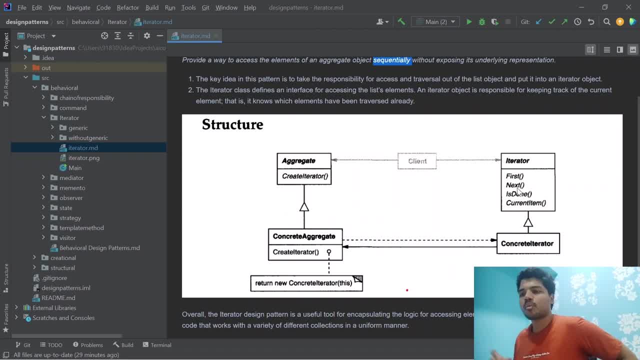 eastern current item. let's say, we'll park a set, So the most important function called next function and has next function Is any, is any object is there? and if it is there, just give me the object. So next and has next. So, uh, there are like multiple, multiple concrete iterators, uh, which will implement the 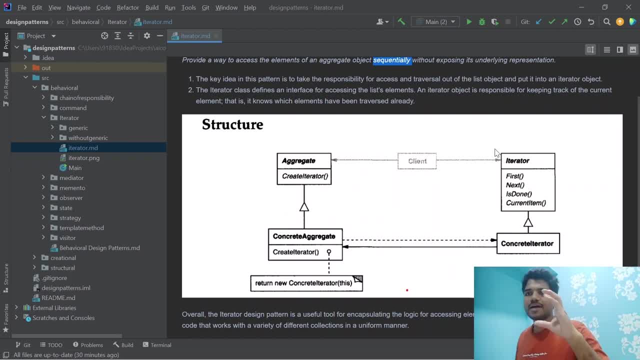 iterator and uh whenever we have an object, let's say aggregate an object. So we will basically uh, at last it has a function called iterator function. There we will call the concrete iterator by passing our complete object. So concrete iterator will basically take care about. 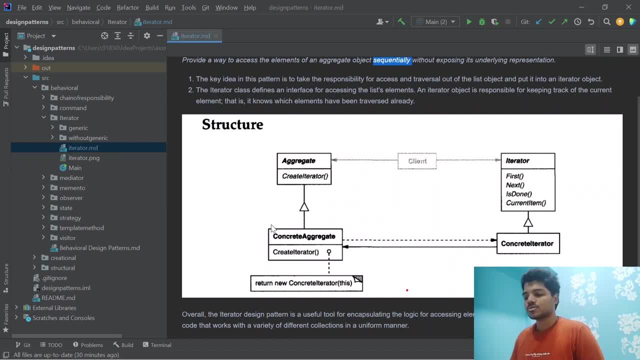 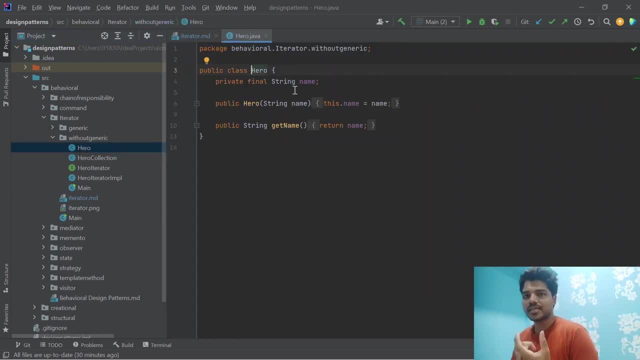 like uh, uh, how this next and has next will work. So let's see, like uh, our, without generic. Let's say I have a, I have a hero class, which is basically, it has a hero name. So I have a hero collection where I have list of heroes. I'm adding hero, uh, and also, at last, this: 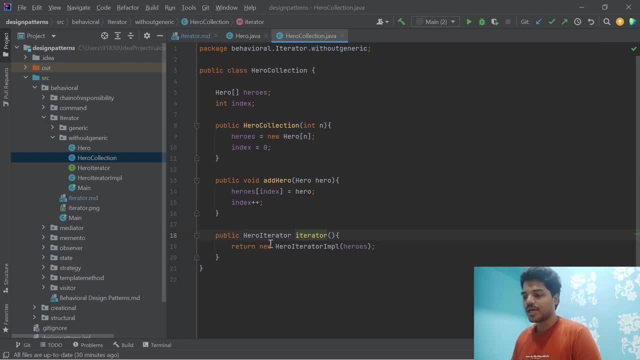 is the most important way. I'm most important thing. I have an iterator function where basically I'm handing over, I'm passing the iterator function, I'm passing the iterator function, I'm passing the complete hero object into this hero iterator IMPL So that accessing will be taken care by. 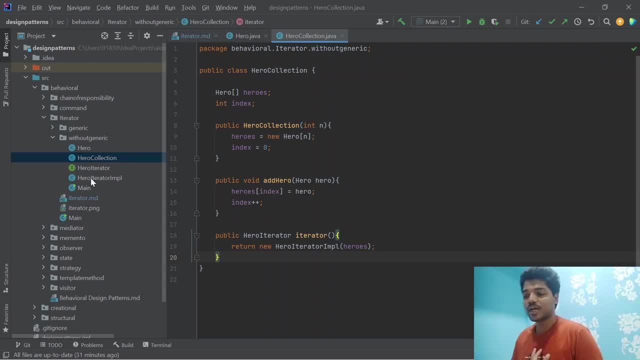 accessing or traversing whatever you say will. it will be taken care by hero iterator IMPL. So before going into here, iterator IMPL, let's see our, uh, our iterator. Our iterator is basically here. iterator will have two functions: called next and has nest. Next will basically attend. 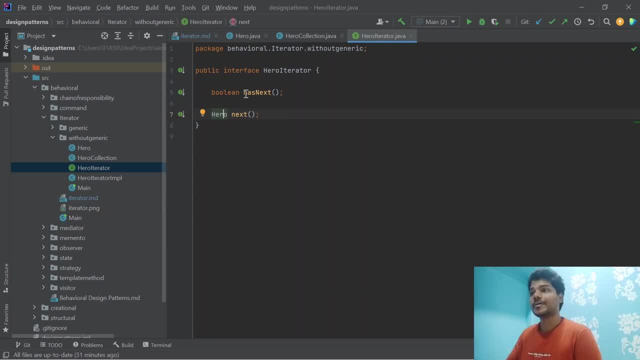 the hero object and has nest, will basically return, whether the, whether um iterator, whether the next object is presented or not, like or that is an end. If it is true, which means like you can, you can still hit traverse, you can still access the object. if it is false, that means there is no. there is no. 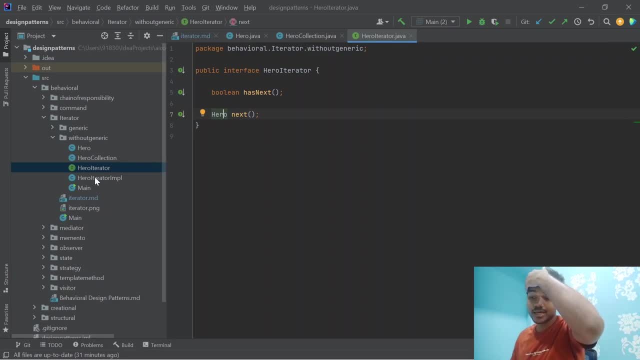 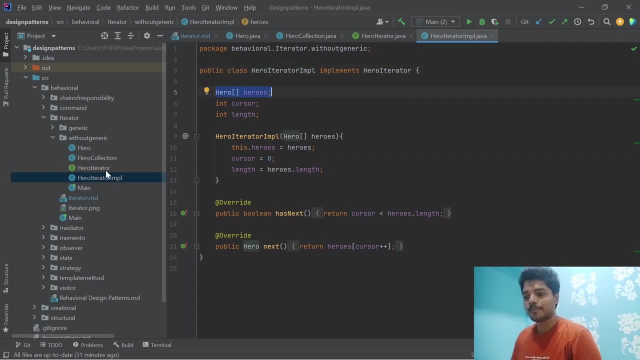 leftover objects still, uh are there like. So now let's see the our main thing, called here iterator IMPL. In the hero iterator IMPL we have like a heroes object, So whatever, uh, whatever data passing by hero collection, we just simply uh copies those things. uh, this dot heroes equals the heroes, Our 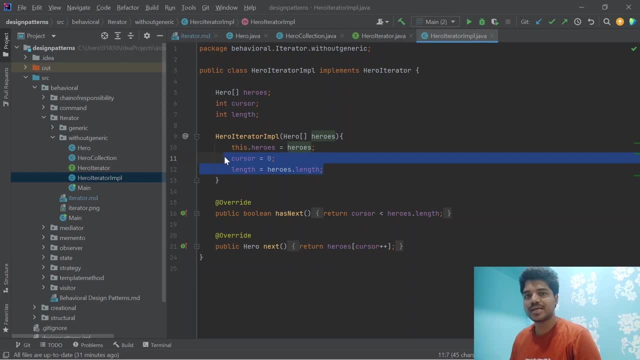 initial cursor is zero. We have total length, So these two will help to check. the has next value For cursor is still less than the heroes of heroes dot length, which will heroes are there In the next uh function. I will just simply returning the initial cursor is zero, right I'm? 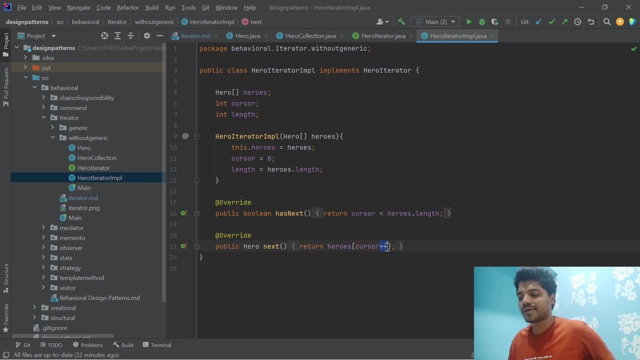 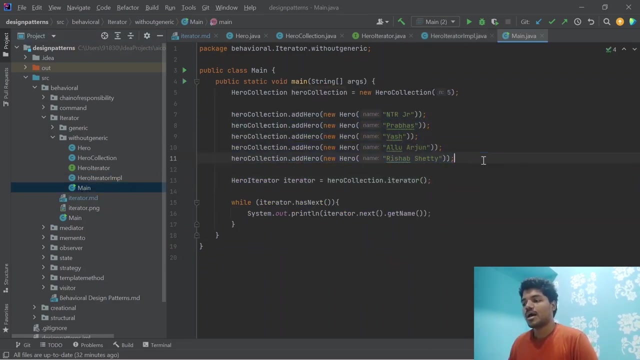 just treating the cursor first, first hero, and I'm incrementing, So happening sequentially and taking care the complete traversal of object. that's where iterator will work like. So now let's see the main program. So I'm adding the heroes, our global star, interior, junior and 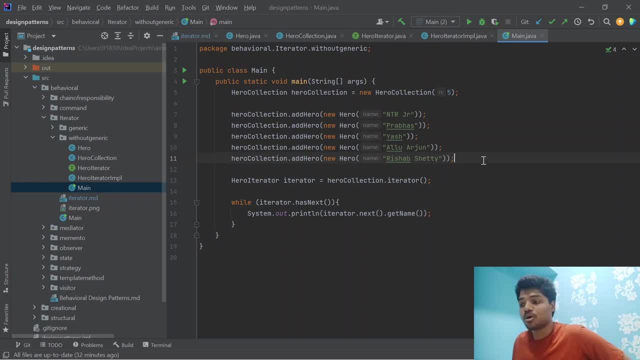 our pan india star preboss and our sboss and our allurgen and reserve citizen. So we have added like around five heroes and I need to traverse right. So I was just passing this uh operation to iterator function. So now iterator function will basically transfer the complete heroes. object: 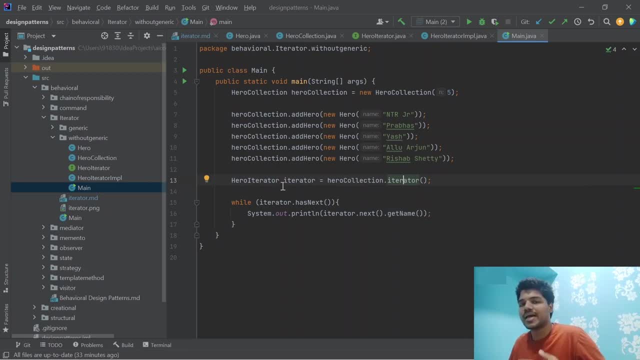 into the hero iterator, IMPL, So, which is basically uh implements by the hero iterator, right? So in the first time I was performing has next, if it is has next, I was getting that, I was uh taking, I was getting the hero and from that hero I was printing the. uh I was, it was getting the. 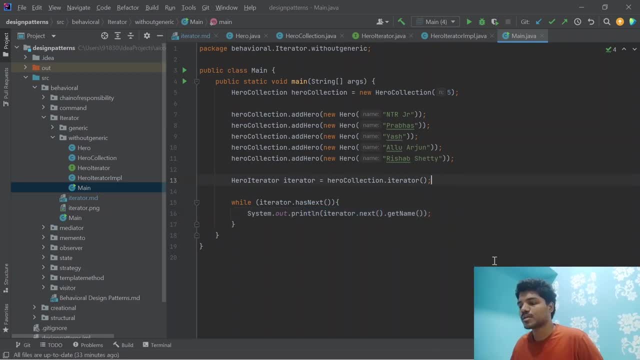 hero object. right from the hero object I was getting the name of the hero. So when you run the program it will print sequentially. That sequence is the most important: Yeah, so you got like india, like preboss, yes and allurgen. and so it. it was printed sequentially. 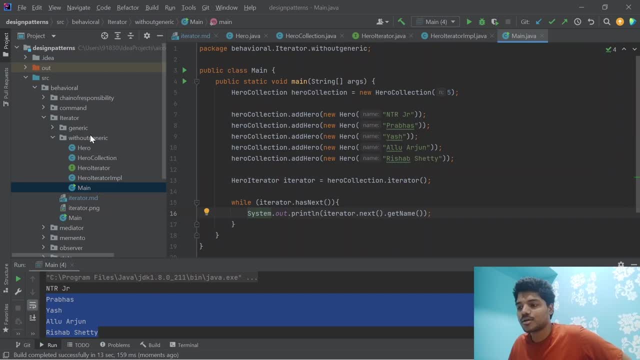 So now let's see like this is like without generic. So here you can only use this one for, only for strings. Let's say, you want to use this one for integers, You want to use this one for float values. how you will do. 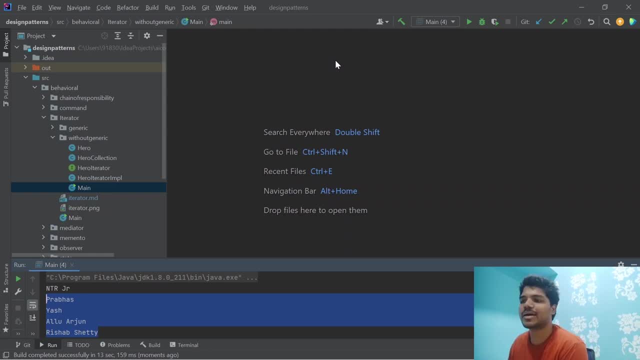 That's what generics will come here. Here I'm explaining one more example, but that's you already learned the iterator concept through this, through the example we just learned. So this is generally more of more of like how we define dynamic input, like 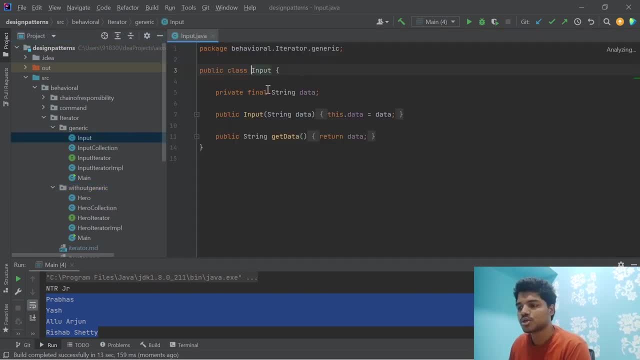 Instead of hero, hero, hero array I was given as input, So input has like string data and input has a collection. It will take the objects. It is not restricting to take the heroes. So, and here I'm passing the heroes in the input: IMPL. 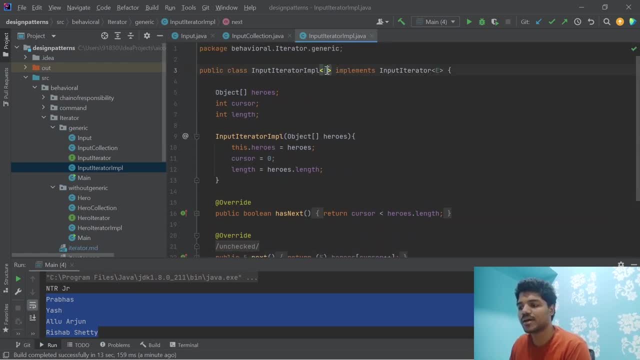 So here the return type is basically the whatever. whatever we want to invoke. It can be either, Let's say, either heroes or it can be either some other object. It can be either some other object. whatever object we should give, it will take like: but 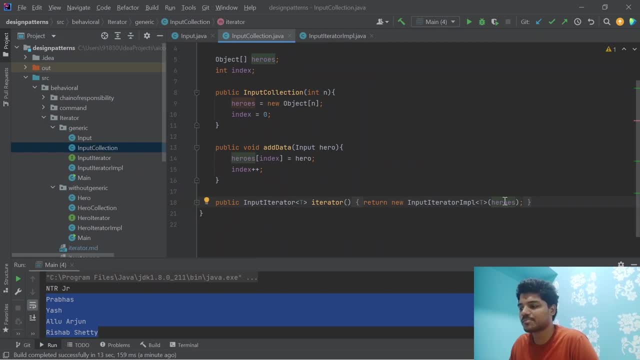 ultimately it was doing the same thing, like in the input collection it is passing the complete heroes information. So here also, if you see that I was giving, I was giving, I was passing the object like it can be any object, either heroes or either heroines, or like directors or like producers. 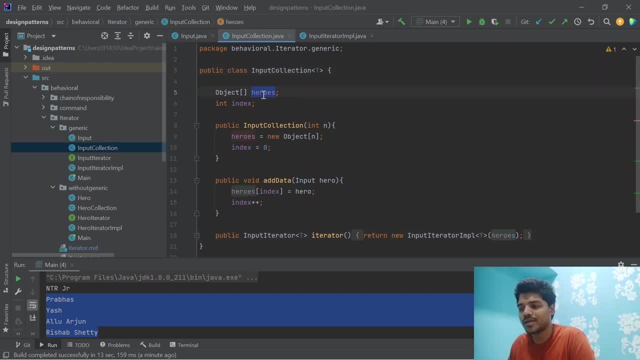 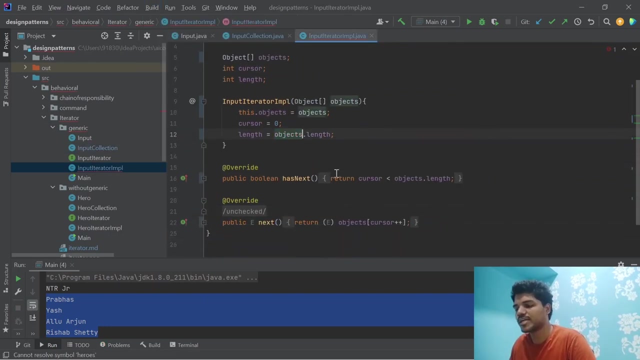 anything like it should take So. So here it should not be heroes, because I just copied like a same thing. I have forgot to change things like: here you can mention objects, I'll do the thing once again. No, he'll see, he'll become even more generic in the next one. 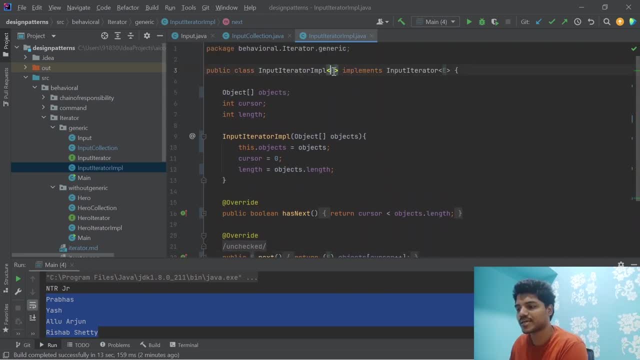 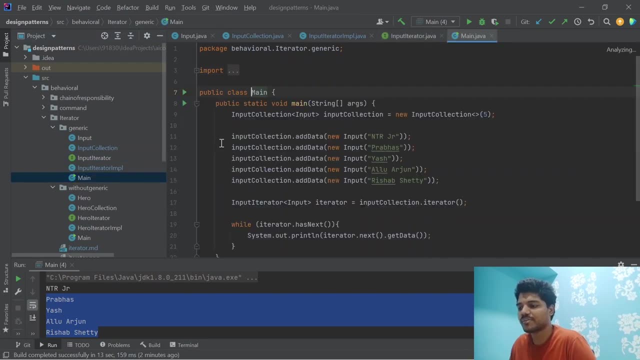 So it will. it will give the return type of E which we are already passing E. So in the input iterator we have we're taking an E and we're returning an E. This can be declared dynamically in the main function. If you see main function here. I was given an input as string. 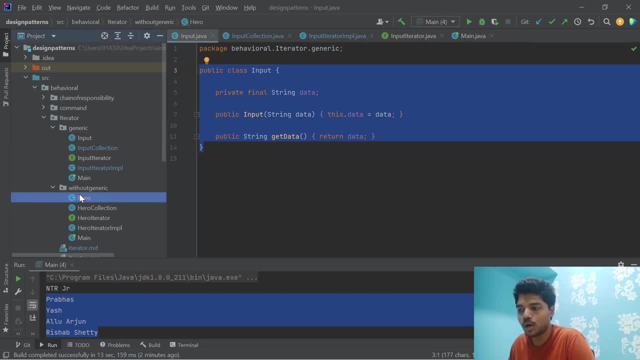 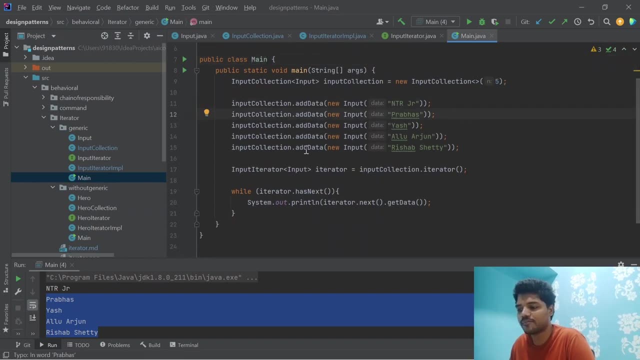 I was giving passing this one. You can simply pass the hero object also. It should give the output like: So here I'm adding: like Indian Junior Prepa, everything same. So it was through iterating. it was giving the output like: so everything works as same. 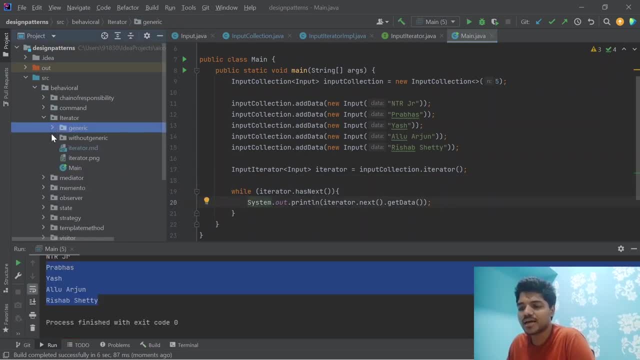 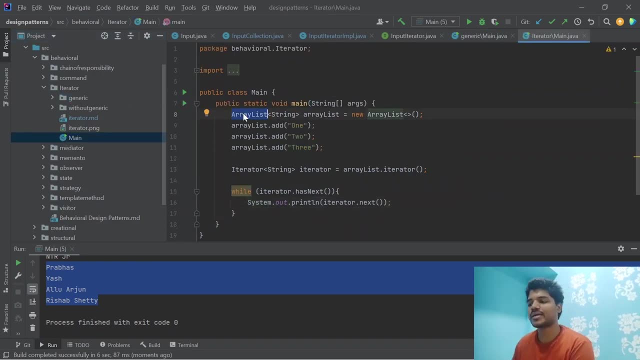 but this is like even more generic. So at last we will see the how existing iterator object. So if you are working with ArrayListRate, you might add all these things Here in the input iterator. you can see the output. So if you are working with ArrayListRate, you might add all these things. 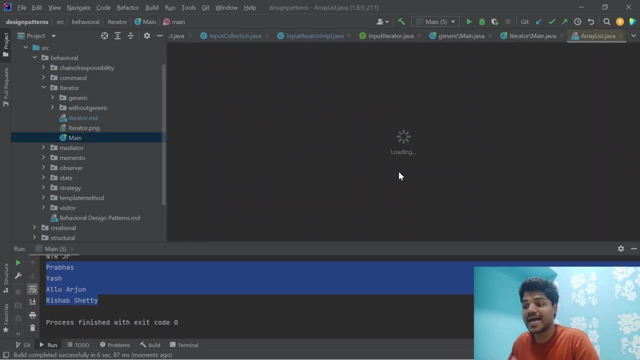 Here in the input iterator you can see the output. So if you are working with ArrayListRate, you might add all these things Here in the input iterator. you might add all these things. You can see the result In ArrayList. it has default iterator present in ArrayList. 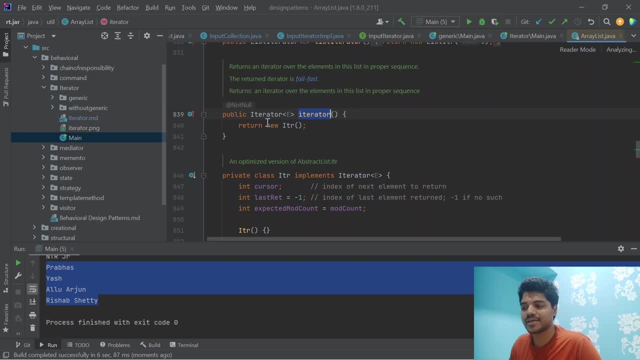 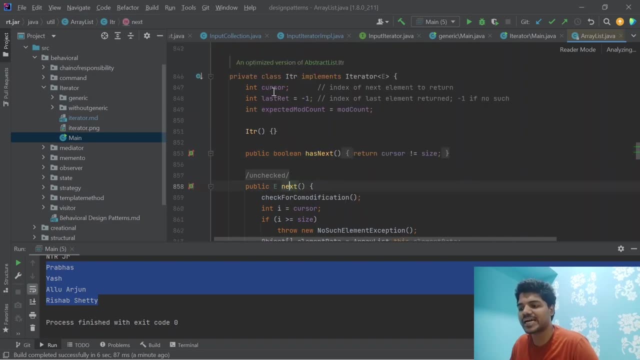 It is also doing the same thing. It is creating a new iterator object and transferring the job to iterator Iterator has the has, next and next. So here also exactly doing the same thing. what we just do So cursor not equal size.